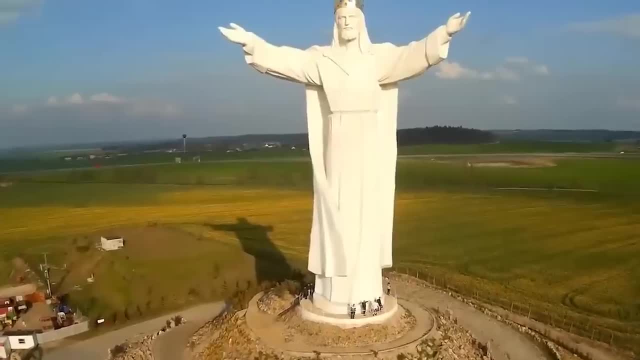 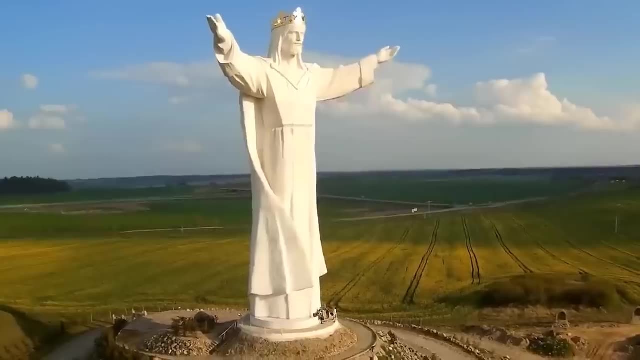 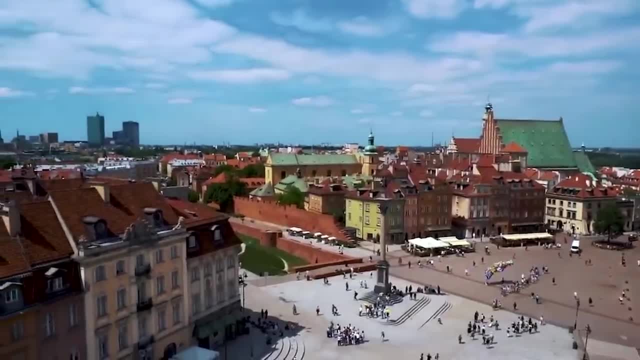 The name Polanyi means people living in Poland. The name Polanyi means people living in open fields. It's indeed a fitting name for a country that has such vast and beautiful plains. Number 5. Did you know that Poles have their own version of Fat Thursday? 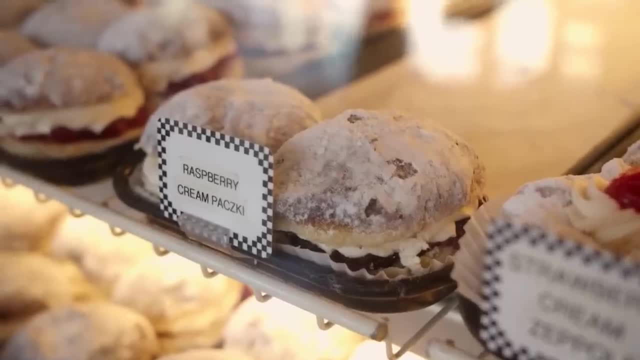 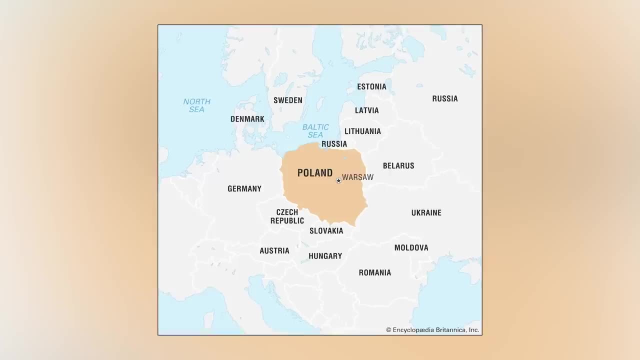 Tlusty Kwartek is a way where Poles indulge in eating donuts or paczki. Millions of these sweet delights are consumed across the country on this day, Number 6.. Polish, known as Polski, is spoken by approximately 40 million people in the world. 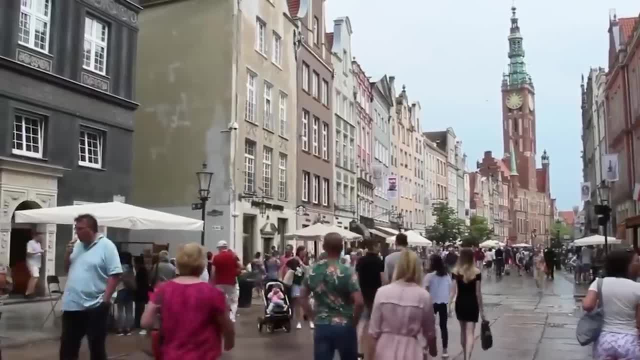 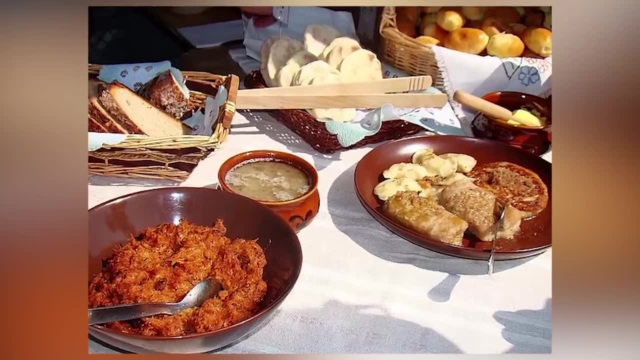 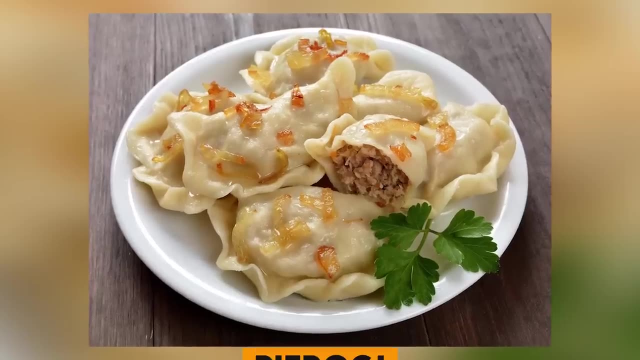 The language has a reputation for being one of the most difficult for English speakers to learn, due to its complex grammar and pronunciation. Number 7. Polish cuisine is hearty and rich in meat, vegetables and herbs. Poland is famous for its sausages, especially the kielbasa and the beloved pierogi. 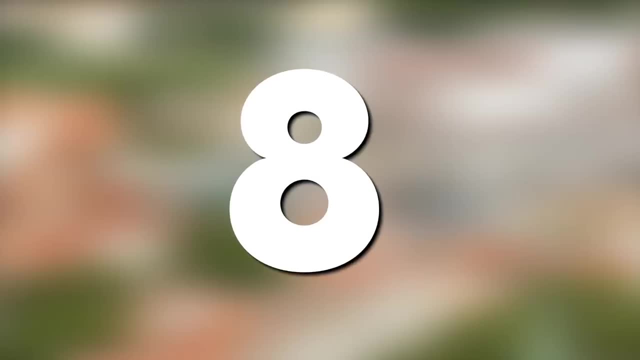 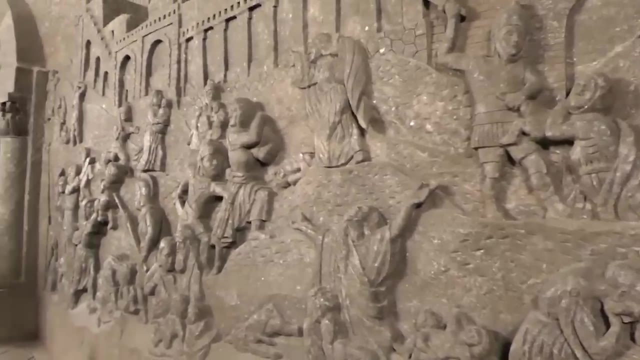 a type of dumpling filled with various ingredients. Number 8. Poland is home to one of the world's oldest salt mines, the Wiliczka salt mine. It's so old, in fact, it has been producing table salt since the 13th century and is now considered a. 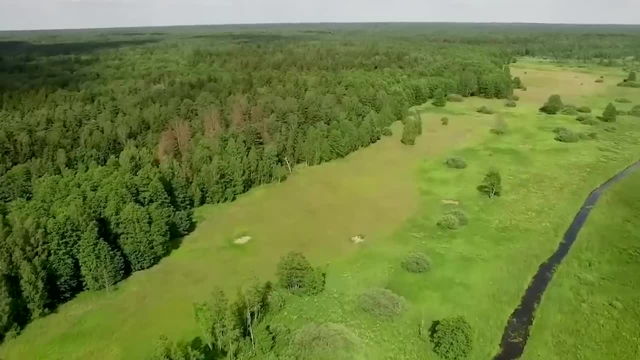 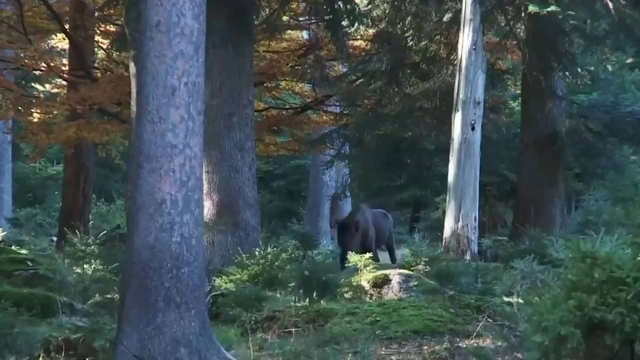 UNESCO World Heritage Site Number 9.. The Poles love their forests. In fact, over 30% of the country is covered by forest. It's no wonder that Poland is home to Europe's last and largest remaining parts of the primeval forest, the Bielowiza forest. 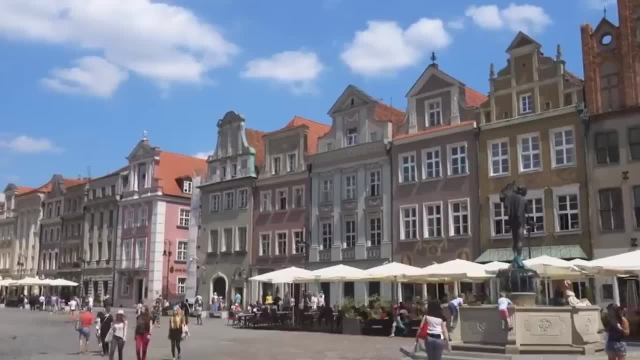 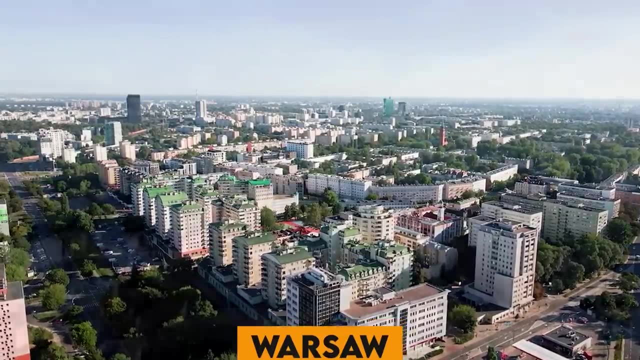 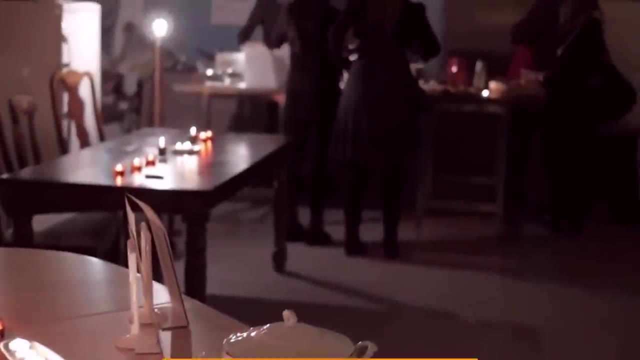 Number 10. Poland, as of the most recent United Nations estimates, has a population of approximately 41.48 million people. The capital city, Warsaw, alone, is home to 1.8 million residents. Number 11. A unique Polish tradition is Andrzejski, or St Andrew's Day. 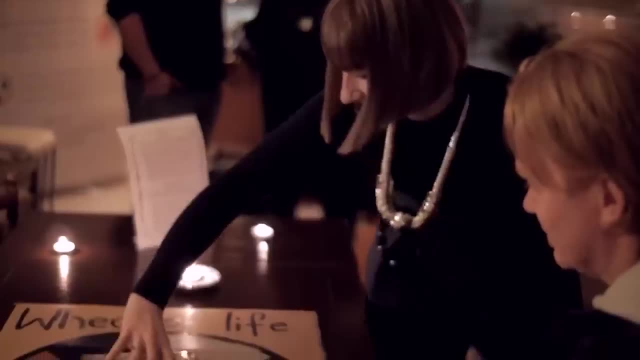 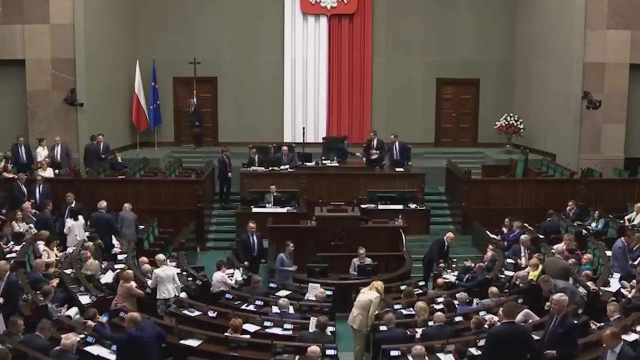 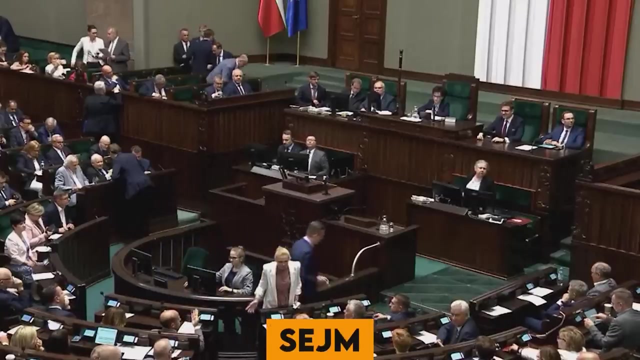 celebrated on the night of November 29,, involving fortune-telling games, especially for young women seeking to predict when and whom they will marry Number 12.. Poland is a parliamentary republic, which means the president is the head of state and the prime minister is the head of government. The Polish Sejm, a component of the parliament. 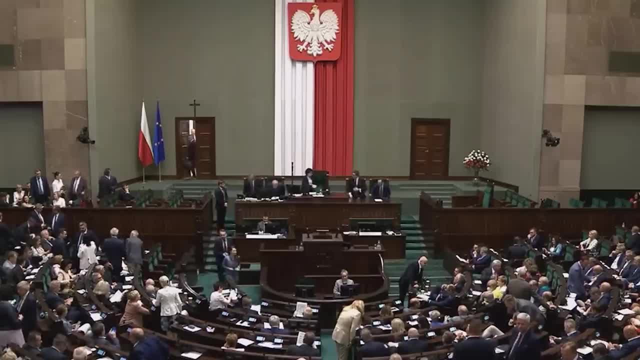 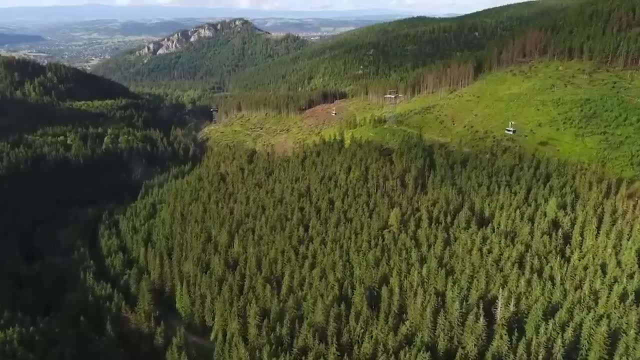 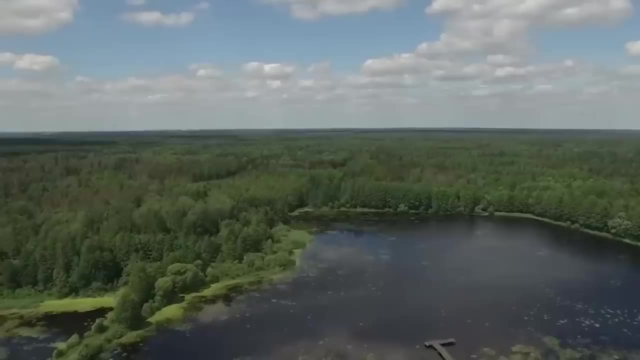 has been in existence since the 15th century, making it one of the oldest parliamentary in the world- Number 13.. The beauty of Poland's landscapes is complemented by its diverse wildlife. Poland is home to the European bison, a species that was brought back from the brink of extinction and can now be found in the Bielowiza. 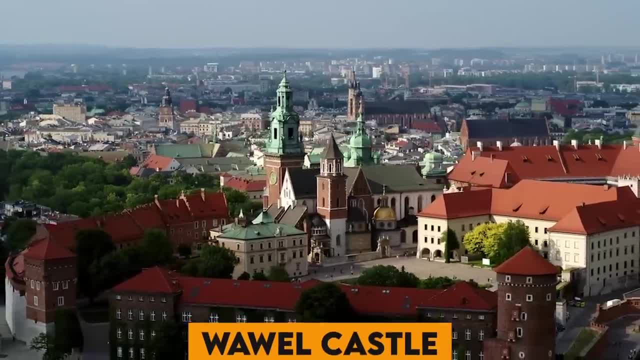 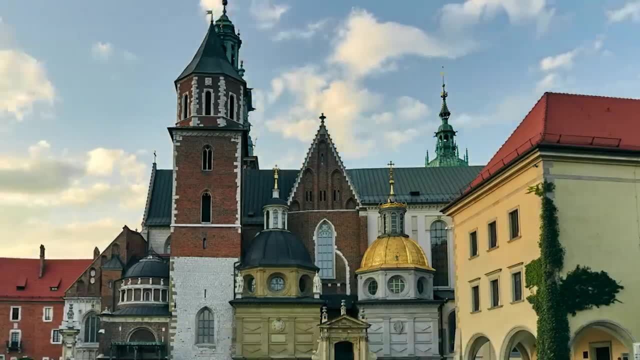 forest- Number 14. Poland's Wawel Castle, a beautiful architectural gem in Krakow, is a symbol of national pride and was the residence of the kings of Poland- Number 15. The Polish flag is composed of two horizontal stripes of equal. 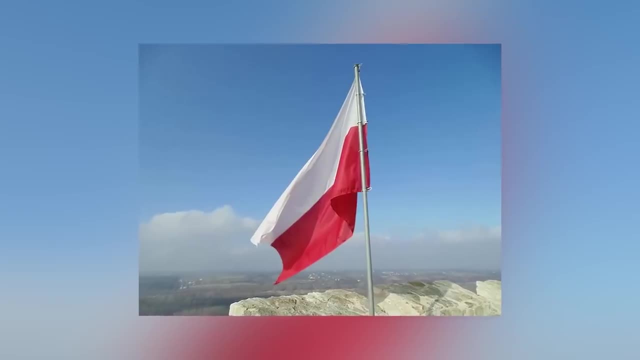 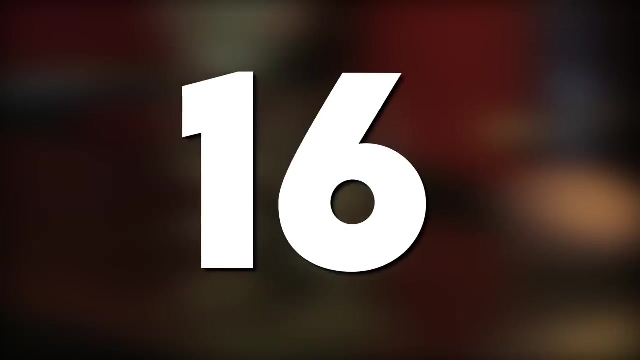 width, the upper one white and the lower one red. These colors, officially adopted in 1831, are of heraldic origin and represent the two national colors Number 16.. Poland is known for its love of vodka, and the tradition of vodka production dates back. 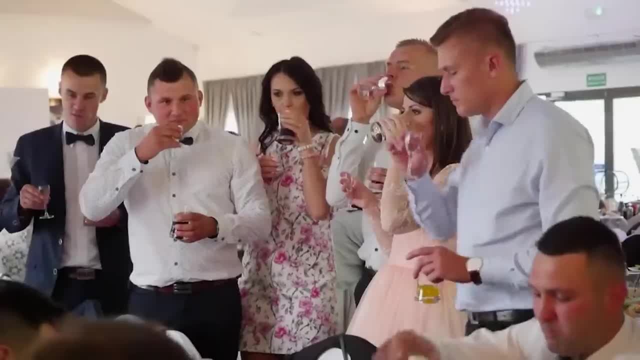 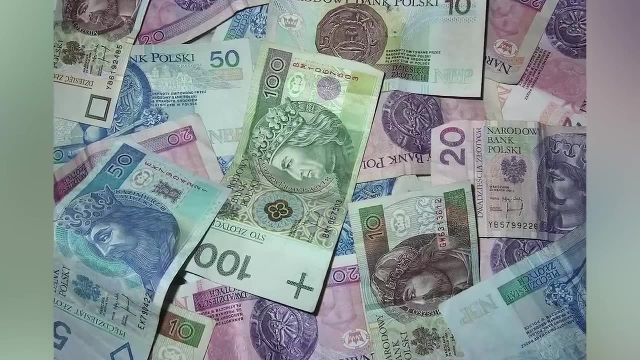 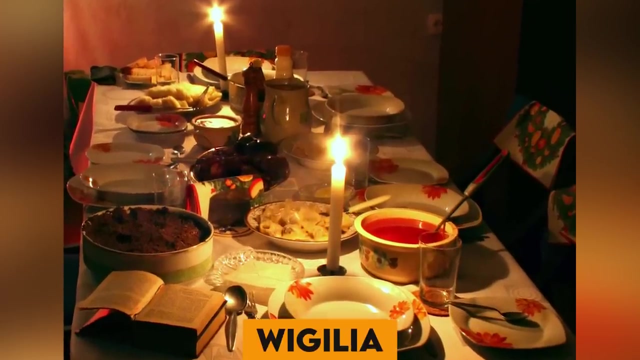 over 500 years. A typical Polish toast is nadzrowi, which means to health, Number 17.. The Polish zloty is the currency of Poland. The word zloty is a Golden Slavic word used to mean a certain thing. The Polish flag is a symbol of the Polish tradition. 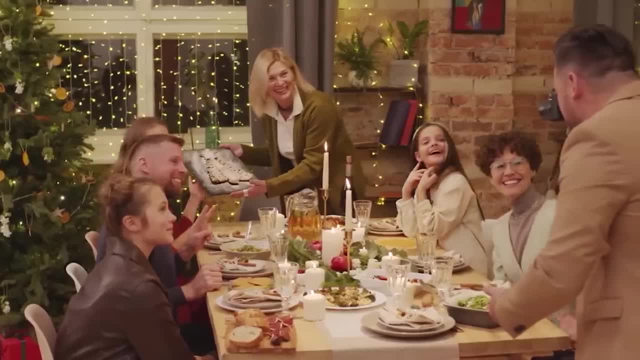 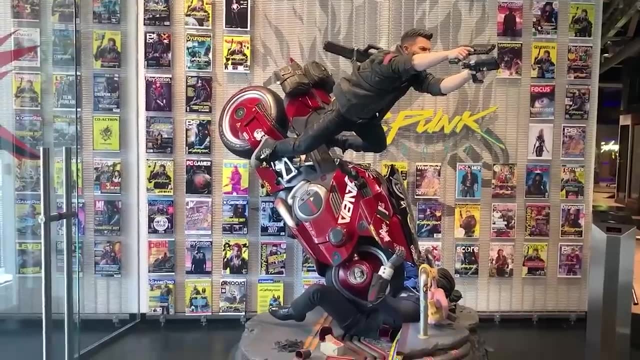 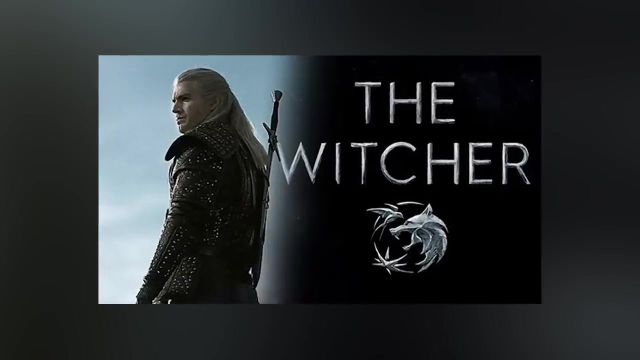 Number 18. Poles have a unique tradition called Wiglia, celebrated on Christmas Eve. An extra plate and seat are always left empty in case a wanderer or even a spirit stops by in need of solace. Number 19. Poland is famous for producing some of the world's best and most popular video. 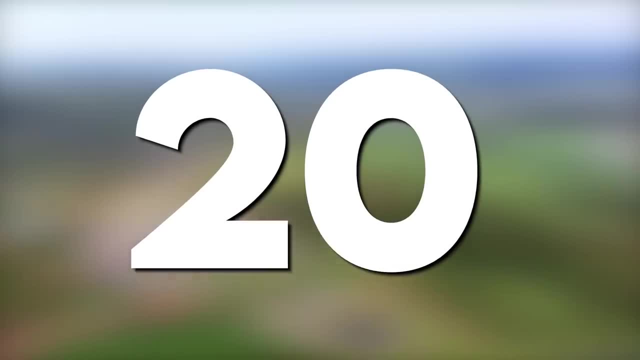 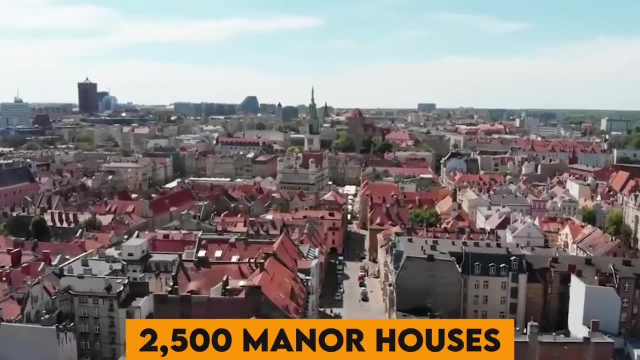 games. Companies like CD Projekt, creators of the widely acclaimed Witcher series, are based in Poland- Number 20.. There are over 500 castles in the country and 2,500 manor houses. Talk about a land straight out of a fairy tale. Number 21.. 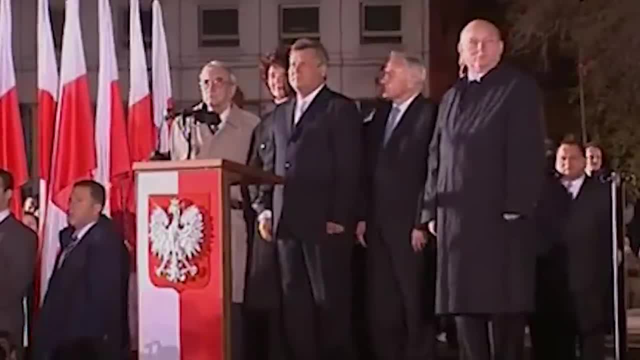 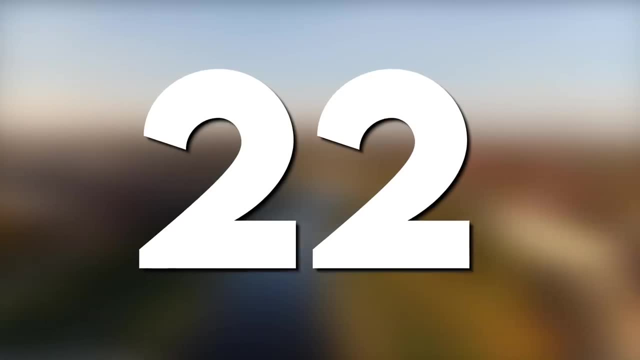 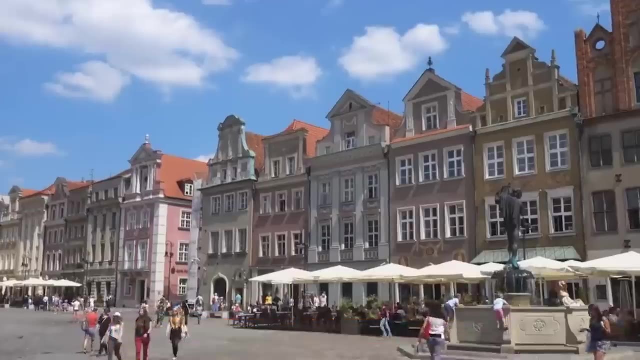 Poland joined the European Union on May 1, 2004,, marking a significant step in its history and signifying the country's economic and political stability. Number 22.. Poland has 15 UNESCO World Heritage Sites. These include the historic centers of Warsaw and Krakow, the Auschwitz-Birkenau concentration camp. 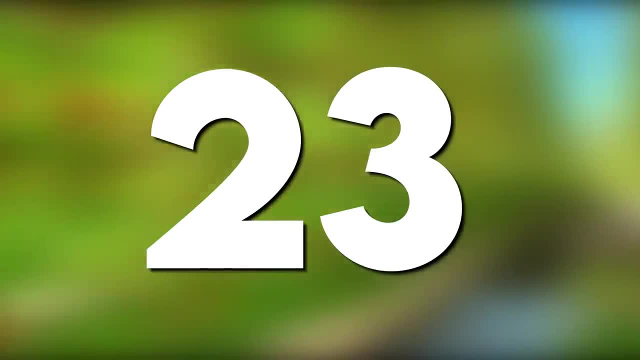 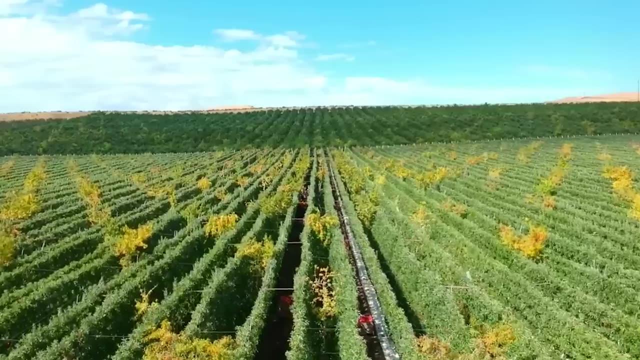 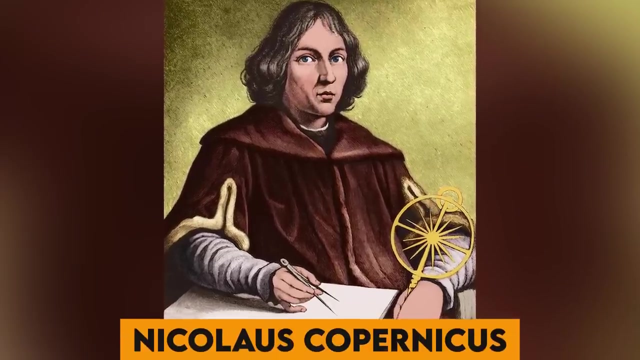 and the ancient Bielowiza forest. Number 23. Poland loves its apples. In fact, in 2020, Poland was the world's largest exporter of apples, contributing to almost 25% of the global apple exports. Number 24. Named after astronomer Nikolaus Copernicus: the Nikolaus Copernicus University. 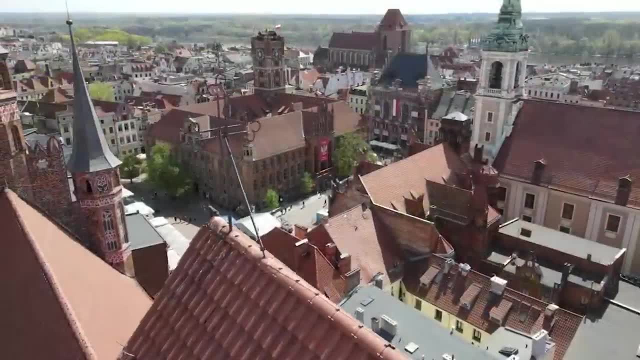 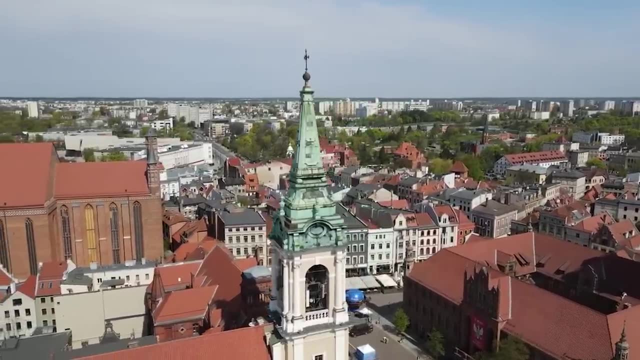 in Toruń is one of the most prestigious universities in Poland. It's named after Copernicus, who was born in Toruń and was the first person to propose that the Earth was not the center of the universe Number 25.. 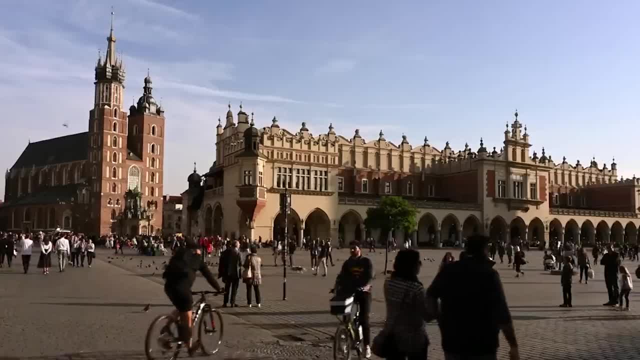 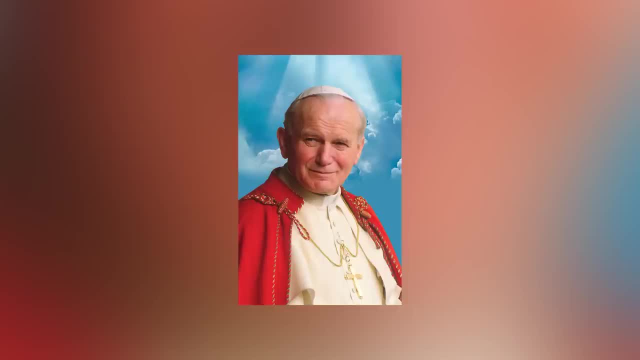 Poland can proudly claim to be the birthplace of many renowned personalities, including world-changing physicist and chemist Marie Curie, legendary film director Roman Polanski and Pope John Paul II, Number 26.. Did you know? Poland has a crooked forest. 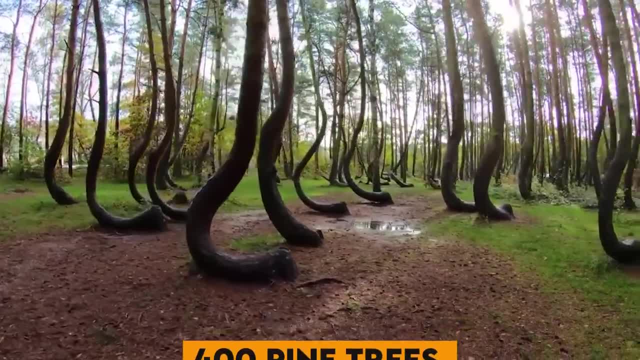 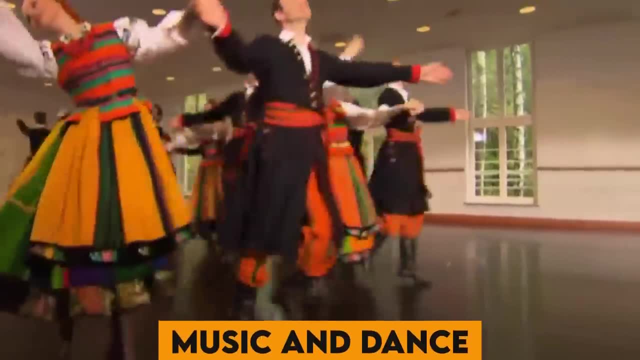 This unusual forest consists of about 400 pine trees that grow with a 90-degree bend at the base of their trunks, Number 27.. Poland has a rich tradition of music and dance, with the mazurka, polonaise and krakowiak being three of the national dances of Poland. 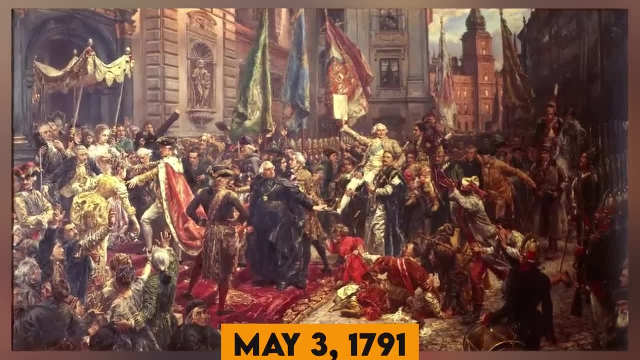 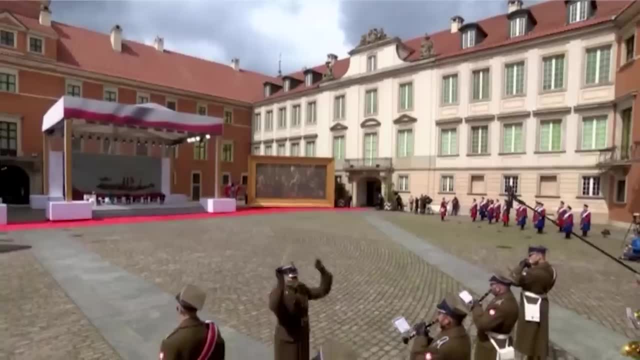 Number 28.. The Polish constitution of May 3, 1791 was the first written constitution in Europe and the second in the world, only preceded by the United States Constitution. It was a significant achievement in Poland's history and the history of democracy worldwide. 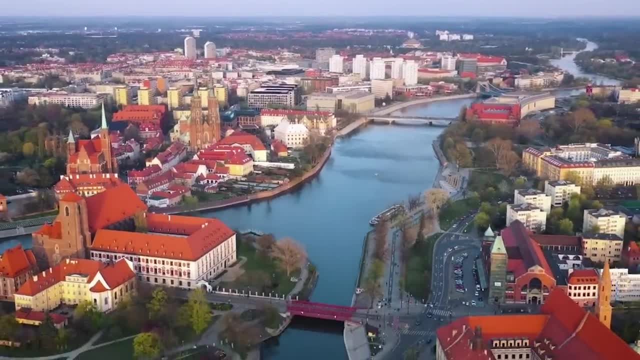 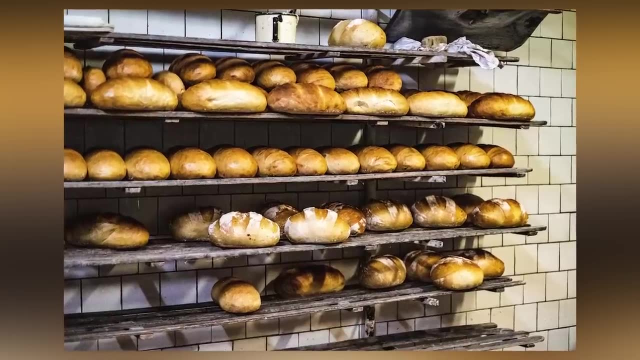 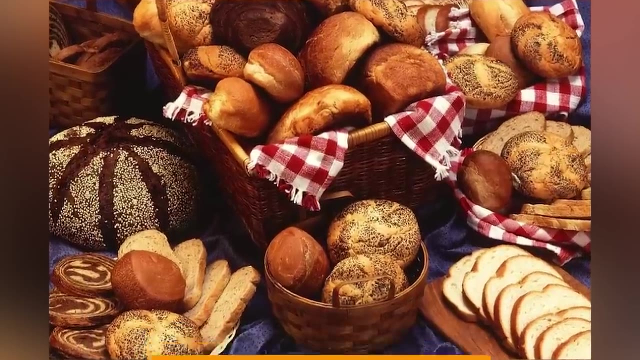 Number 29.. Poland is the sixth most populated country in the European Union and the ninth largest in Europe by area 30.. Baking bread isn't just a routine in Poland. it's an age-old tradition, treasured and carried forward with pride. So much so that when a bread loaf drops, it is customary to pick it up and 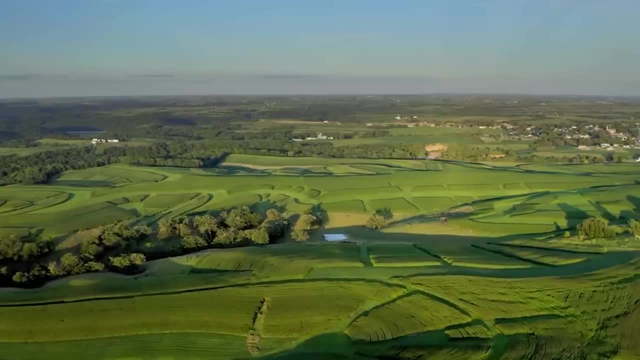 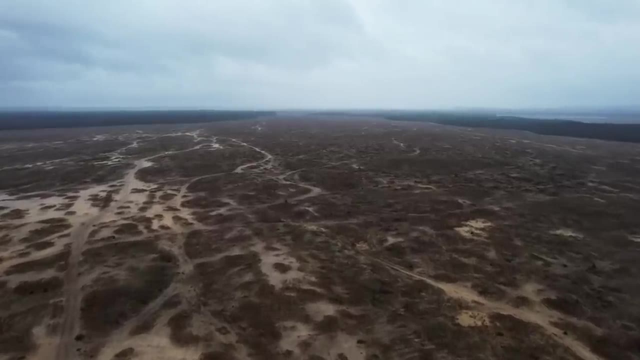 kiss it as a sign of respect. 31. Can you imagine a desert in the middle of Europe? Well, Poland is home to one. The Bledau Desert is Central Europe's largest accumulation of loose sand, in an area away from any sea spanning over 12 square miles. 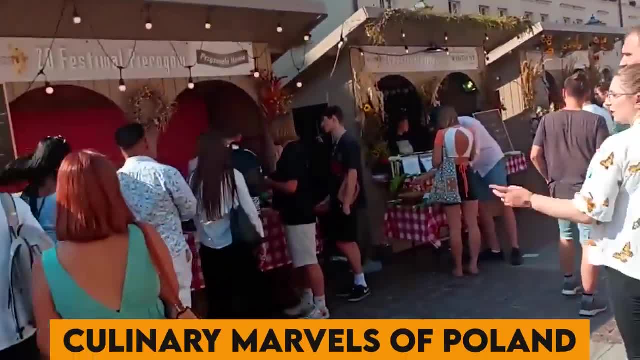 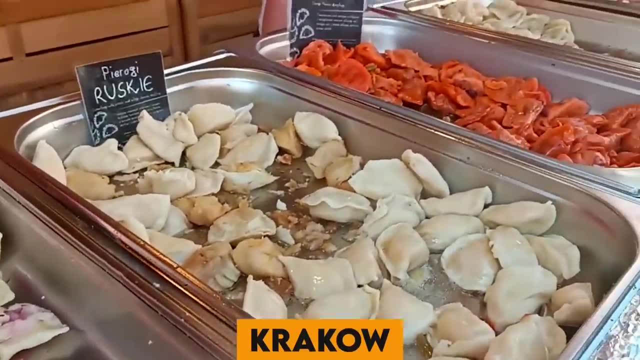 32. Let's dive into the culinary marvels of Poland. Ever heard of pierogi? These delicious stuffed dumplings are a must-try. They're so beloved that the city of Krakow even hosts an annual pierogi festival. 33. The Polish hold a deep reverence for 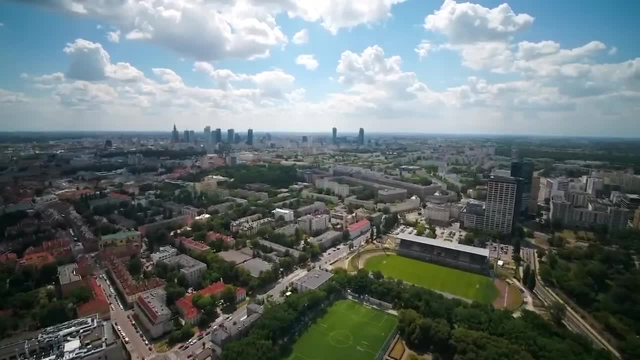 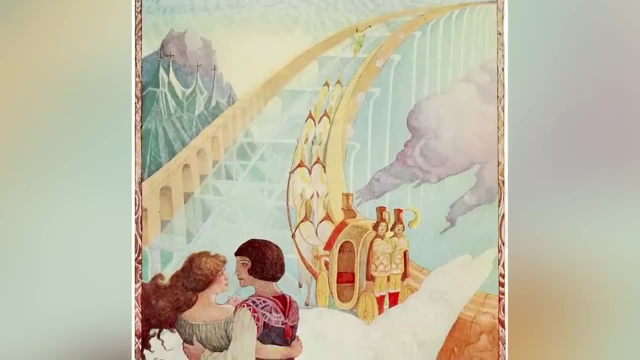 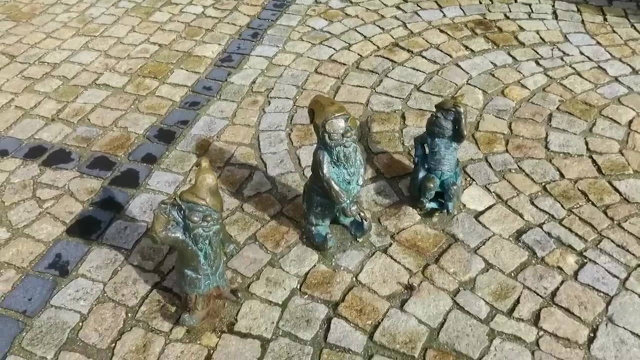 the number three, symbolizing luck and magic. You'll find this love echoed in the structure of the traditional Polish fairy tales, where the rule of three is often applied: Three tasks, three characters or three goals, 34. In the heart of Wrocław City, you'll stumble upon a tiny world of gnome sculptures With over 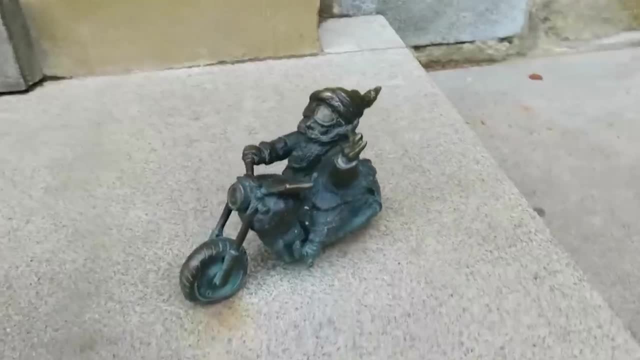 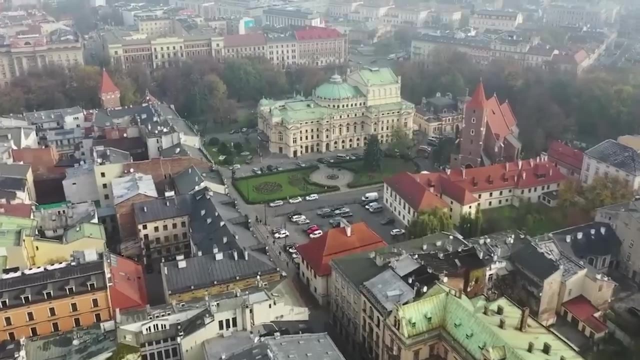 350 dwarf statues scattered across the city. the hunt for these charming creatures has become a fun pastime for tourists and locals alike. 35. Did you know that, with a history dating back over a thousand years, Krakow is one of Poland's oldest cities? 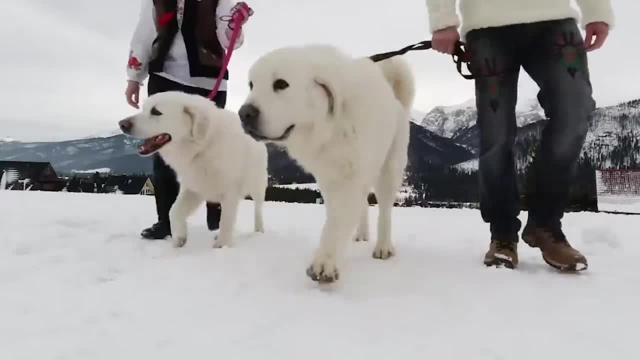 36. The Tatra Mountains in Poland are home to the unique breed of sheepdog known as the Polish Tatra. 35. The Tatra Mountains in Poland are home to the unique breed of sheepdog known as the Polish Tatra Mountains. 36. The Tatra Mountains in Poland are home to the unique breed of sheepdog known as the. 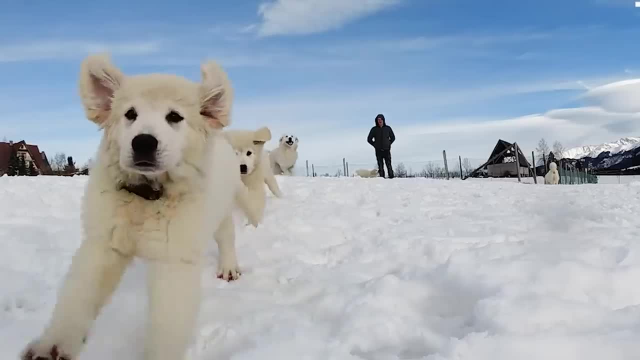 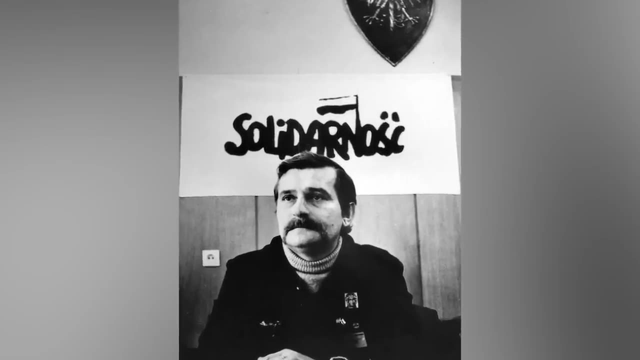 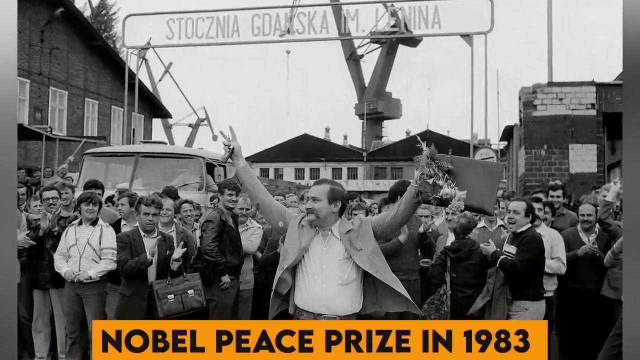 Tatra Sheepdog. These dogs were used to protect sheep from predators in the mountainous region. 37. Lach Walesa, the co-founder of the Solidarity Movement in Poland, played a pivotal role in the fall of communism across Eastern Europe. He was awarded the Nobel Peace Prize in 1983 and later. 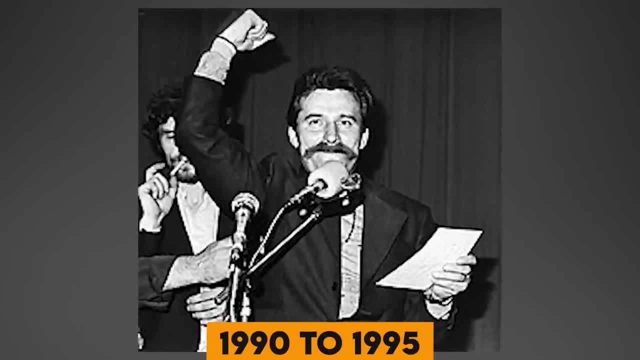 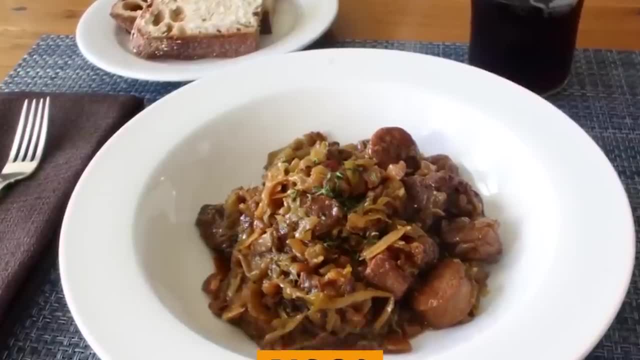 served as the President of Poland from 1990 to 1995.. 38. One cannot talk about Poland without mentioning its hearty traditional stew, bigos. 39. This savoury dish is known as the bigos. This savoury dish is a flavourful mix of cabbage, sauerkraut, various meats and spices. 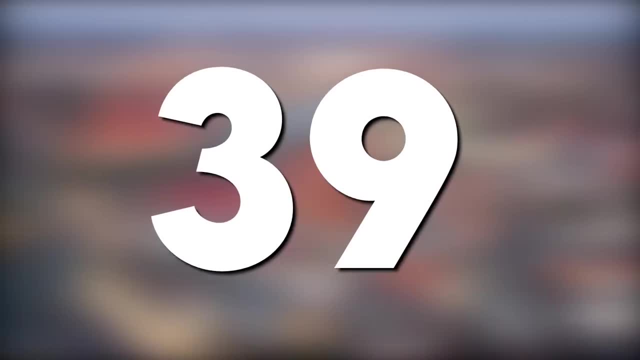 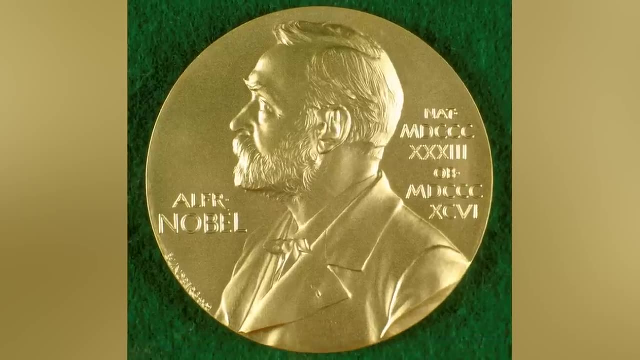 often described as Poland's national dish. 39. Poland is home to 17 Nobel Prize winners, including four Peace Prizes and five Literature Prizes. This country certainly has a wealth of intellect and talent. 40. The world's first oil. 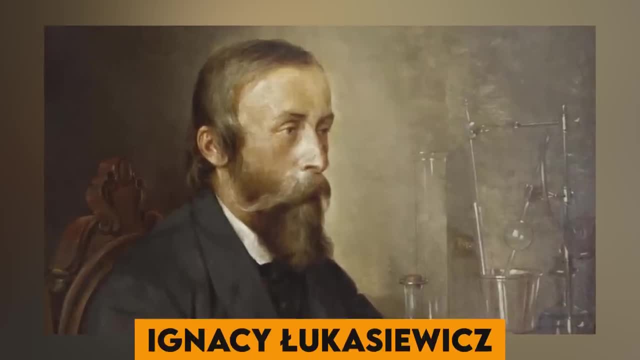 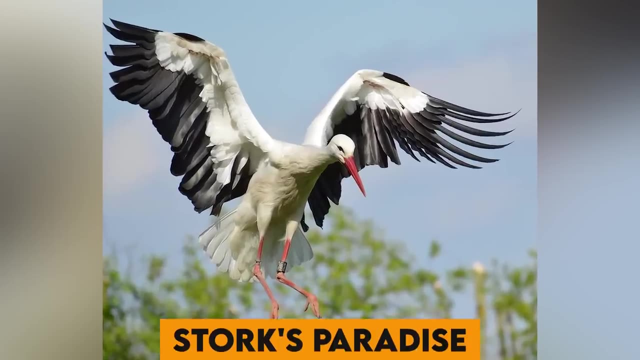 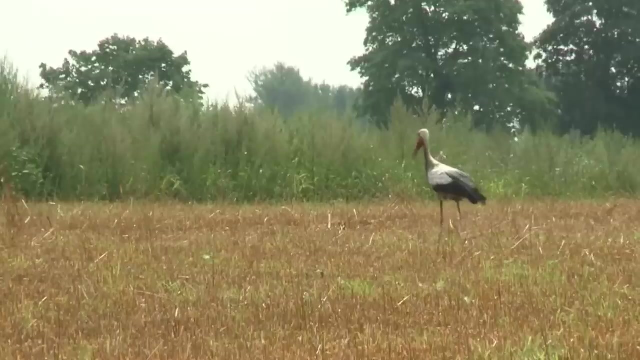 refinery was built in 1856 by Ignacy Lukasiewicz, a Polish pharmacist and petroleum industry pioneer. 41. Poland is a stork's paradise. Nearly a quarter of all white storks in the world nest in Poland during the summer. In fact, the village of Sikowo is known as the European Stork Capital. 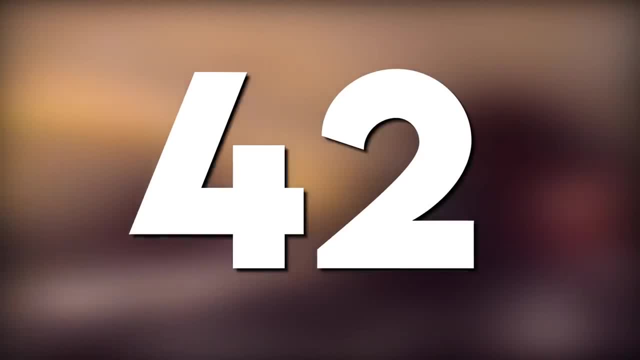 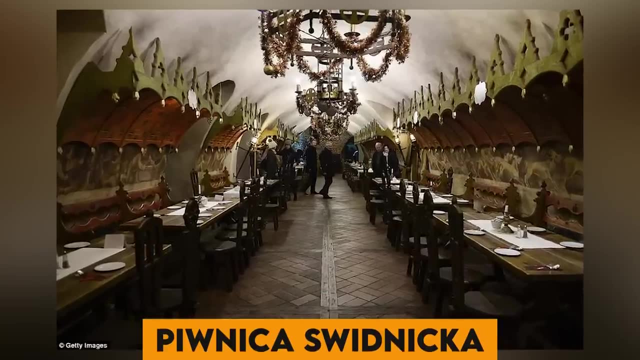 hosting about 40 stork pairs per season. 42. One of the oldest restaurants in Europe is located in Wrocław, Poland, named Pułynica Swydnika, It has been serving customers since 1275.. 43. The first-ever. 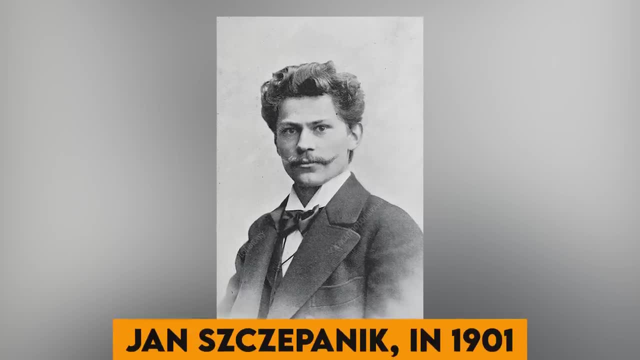 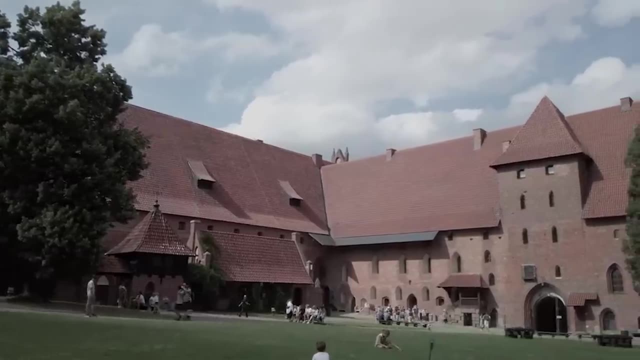 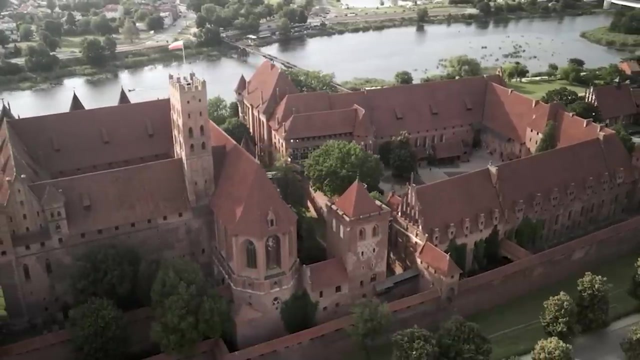 bulletproof vest was invented by a Polish inventor, Jan Sipanek, in 1901.. Number 44.. Not many know that Poland boasts the world's largest castle measured by land area. The castle of the Teutonic Order in Malbork covers over 143,591 square meters.